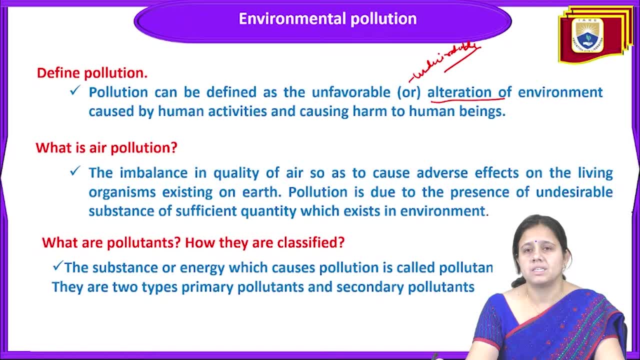 of air or natural of air in human beings. Now this is an undesirable change or an unfavorable change in the quality of air. So the unfavorable or unfavorable change in the quality of physical, chemical or biological properties of air that are not unfavorable orolded in normal living. 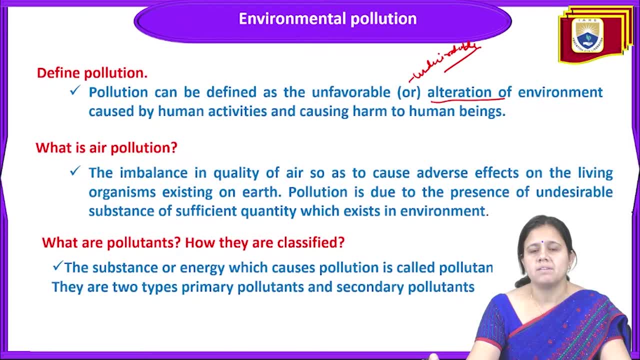 society. So the imbalance or unfavorable change in this environment is called as air pollution. So today we will discuss about air pollution in this language And it should bekan the way of understanding it. change or alteration on the quality of air and so that will be causes adverse. 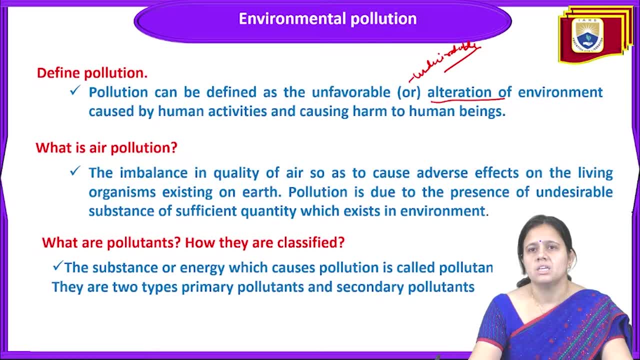 effect on the living organism that is existing on the earth is called as air pollution. so pollution is due to the presence of undesirable substances of sufficient quantity, that is, that exists in the environment means it is the presence of any undesirable substance of sufficient quantity. many means any. 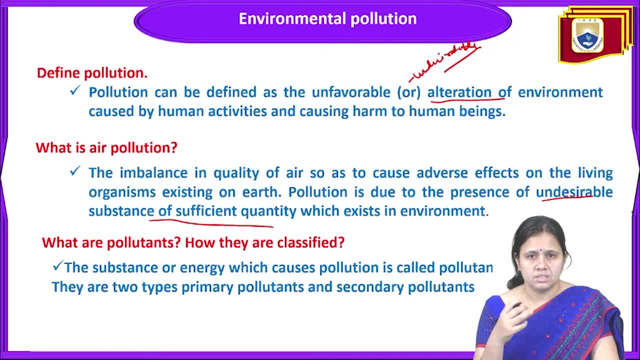 substance that is undesirable, that is not desirable, that is not perfect, that is not good and it is present in a more quantity that is exist in the environment and that will change, that will alter the quality of air, water or soil is called as air pollution and that will be harmful as a in terms of physical 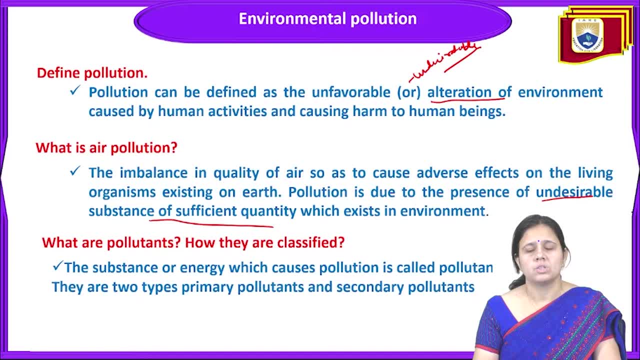 chemical or biological, is called as air pollution. so the imbalance, the basic term logic we can define it. the air pollution is like the imbalance. issa quality of air is to cause adverse effect on the living organism that is existing on the earth is called as air pollution means any unfavorable change or any undesirable change that will be. 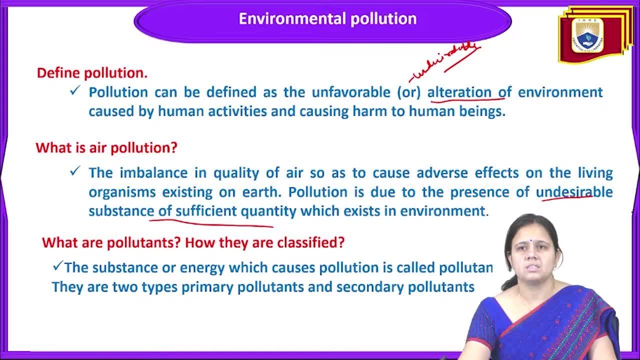 harmful for the living organism that is living on the earth is called as air pollution, and it is due to the presence of any undesirable substance of sufficient quantity that exists in the environment. next term is about what is pollutant and how we can classify the pollutant. so, first of 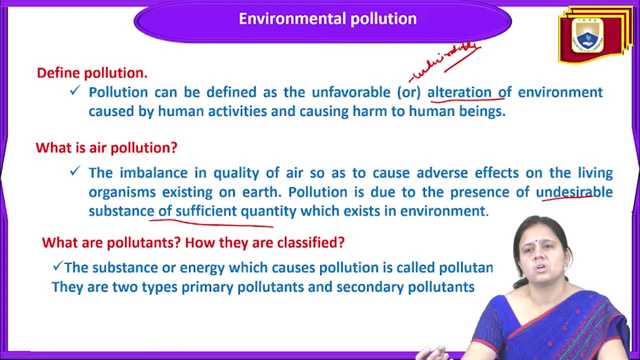 all. pollutant are the substances or energy which causes pollution. is called as pollutant. pollutant are those agents or those things that causes pollution. is called as pollutant. we can define pollutant in a very simple way, that is, those agent or those substance or those energy. 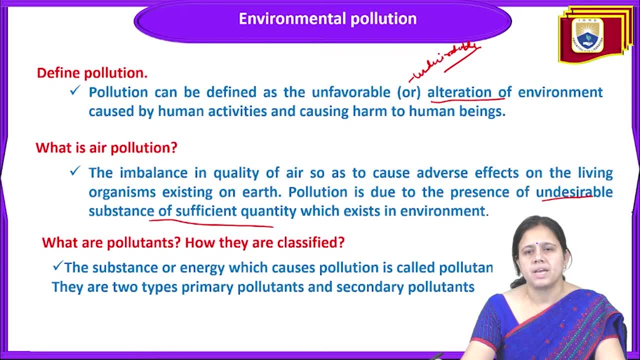 that is causing pollution is called as pollutant, and there are basically two types of pollutant. when we talk about the origin of pollutant, there are mainly two types of pollutant: primary pollutant and secondary pollutant. so we understand the term. pollutant are those things. pollutant is equal to those. 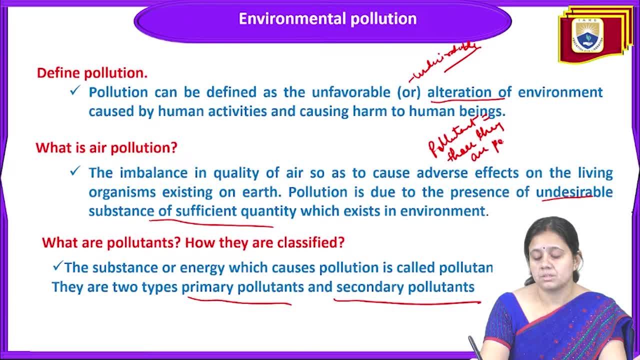 they are polluting. they are polluting, polluting and it is of two type: primary and secondary. primary and secondary, primary pollutant and secondary pollutant. so pollutant or energy which causes pollution is called as pollutant those substance or energy, those things, those, an agent that is causing 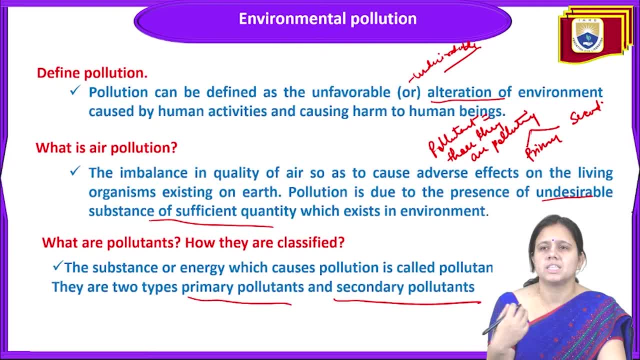 pollution, anything that is causing pollutant pollution, we can say that that is a pollutant particular environment. for in case of air, for in case of air, socks, snogs is the pollutant. in case of water pollution, we can say that the seaways, the silt and the dirty water. 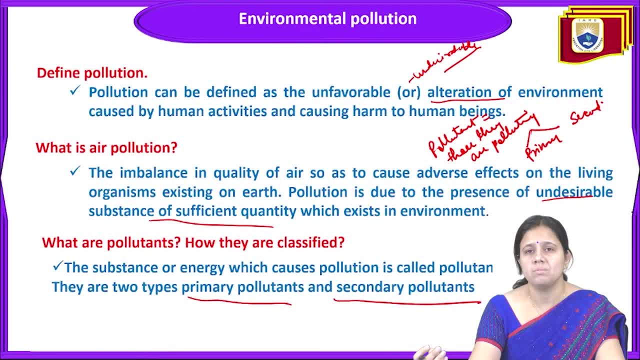 are polluted. in case of a soil pollution, the runoff from agriculture, pesticides, chemicals- all are polluted, so means any agent that is, that is causing pollution is called as polluted. and on the basis of its origin it is divided into two category. first one is the primary pollutant and next is the secondary. 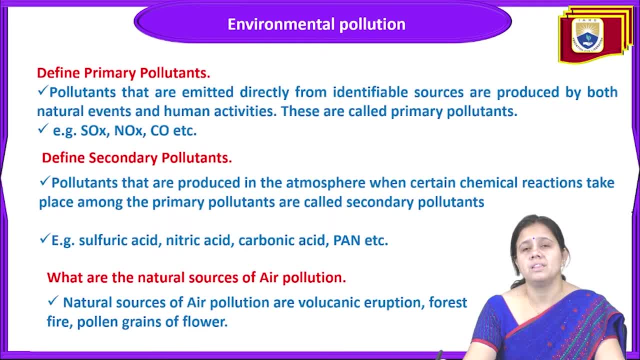 pollutant. now our next thing is like define the term primary pollutant. now we'll come on the topic that is, primary pollutant. what is primary pollutant means? as you already understand the term pollutant pollutant are those agent or those things that is causing pollution. so it is of two type: primary pollutant. 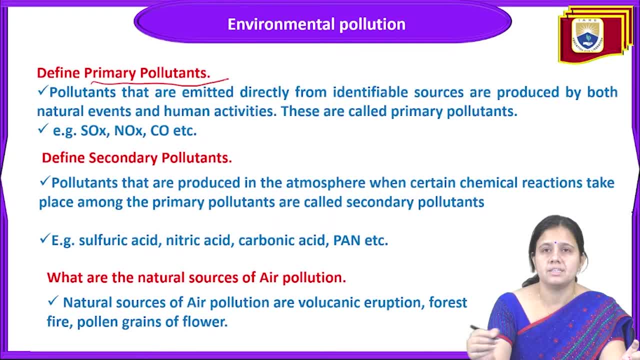 in secondary pollutant, so primary pollutant. define the term primary pollutant so pollutants that are emitted directly from any identifiable source, are produced by both sometimes natural events or by human activity, are called as primary pollutant. means that is, primary pollutant emitted directly from any identifiable source, like carbon monoxide, as we know. 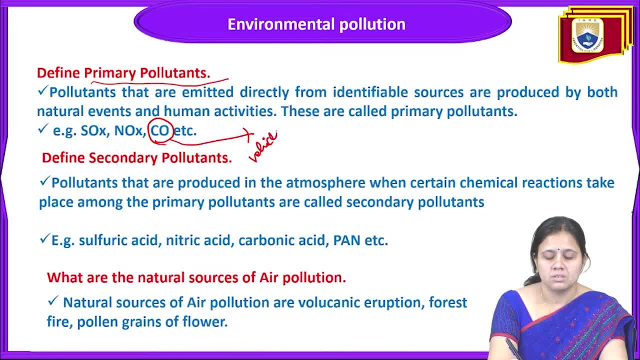 carbon monoxide is coming from vehicle. SOX, NOX is coming from sometimes a factory or industry, so there they can be. identify identifiable source means their source. we know that they are emitted directly from any. identifiable source is called as primary pollutant- pollutant that emitted directly from any. 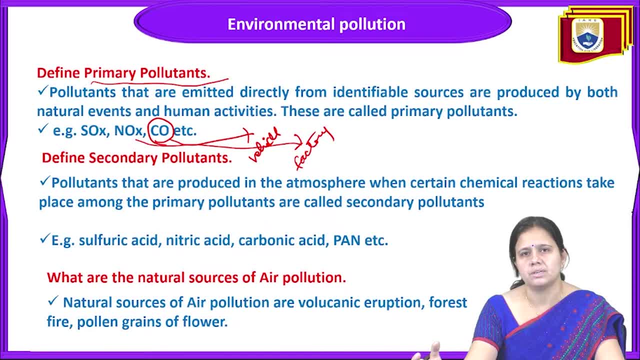 identifiable source is called as primary pollutant. primary pollutant. Next is like a secondary pollutant. So the examples of primary pollutants are SOX, NOX, carbon monoxide, SOX, NOX. we know that that is emitted from the industries. 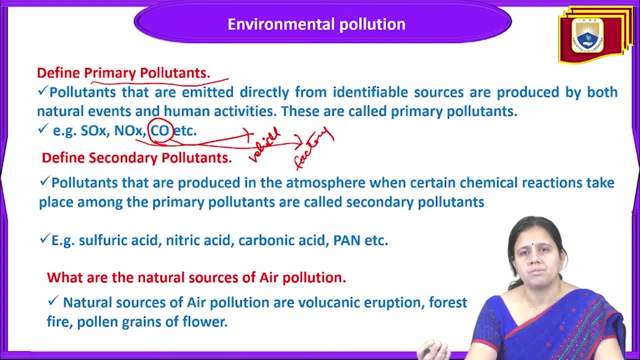 any thermal power plant and carbon monoxide is coming from the vehicles also. So their source- they are directly emitting from any source and their source we can identify- is called as primary pollutant. Next is secondary pollutant: Pollutants that are produced in the atmosphere when certain 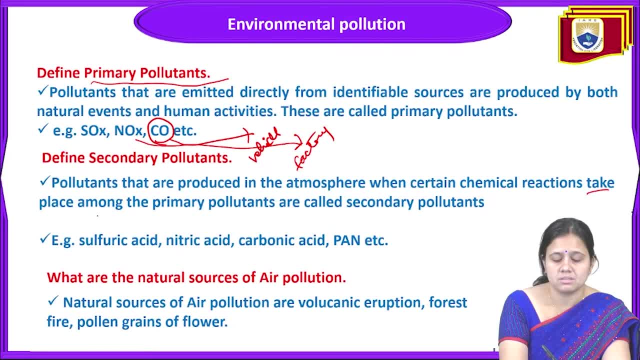 chemical reaction takes place among the primary pollutant means any chemical reaction will take place among the primary pollutant is called as secondary pollutants. Means that will be that will be happen within a with a certain chemical reaction that will be taken place by among the reaction between two primary pollutant is called as secondary. 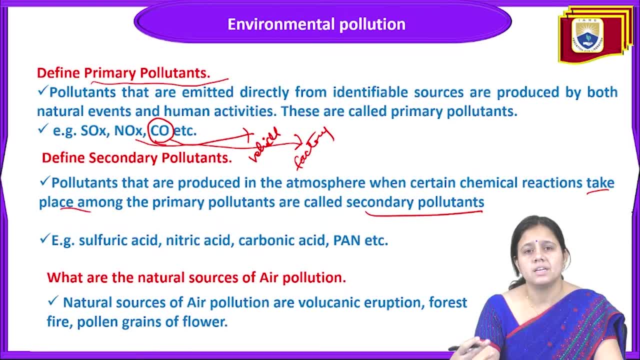 Pollutants, secondary pollutant. we can define it as, like the reaction or some chemical reaction happen between two primary pollutant and the next product will be formed is called as secondary pollutant, and the example for some secondary pollutant is the sulfuric acid, H2SO4, nitric acid. 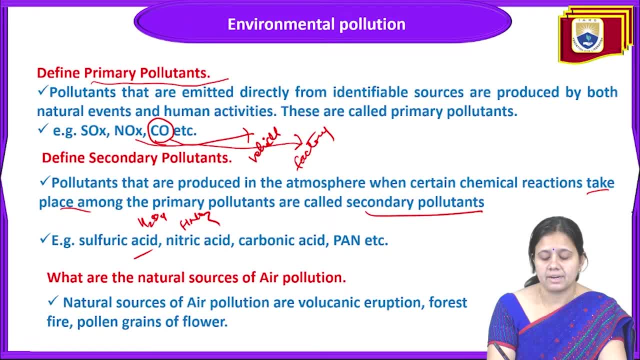 HNO3, HNO3 and the carbonic acid and the PAN. as we know, PAN is the peroxyacyl nitrate. So this is the secondary pollutant. Secondary pollutant, we can say that sulfuric acid, nitric acid, they both. 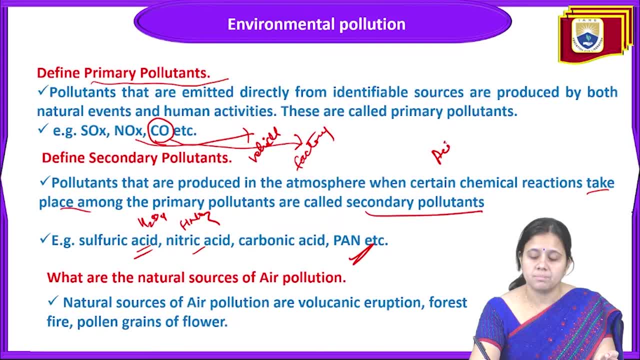 are sulfuric acid and nitric acid. They both are sulfuric acid and nitric acid. They both are secondary pollutant. in case of acid rain, When we know the term acid rain, acid rain is what It is: the rain of acids. So what will happen? and it will containing some concentrated acid like H2SO4. 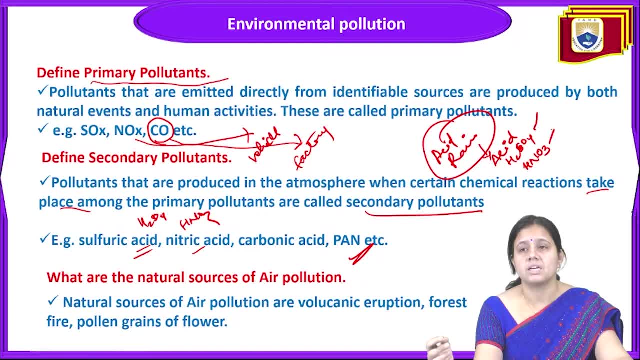 and HNO3. So they both are concentrated acid: H2SO4 and HNO3.. H2SO4 is sulfuric acid and HNO3 is a nitric acid. So these are the secondary pollutant means that will be formed by a. 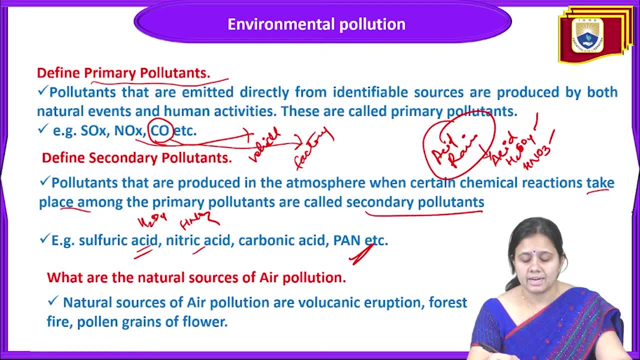 chemical reaction between two primary pollutant like that, PAN is there peroxyacyl nitrate? PAN is also a secondary pollutant. Now next thing, the sources of air pollution. What are the natural sources of air pollution When we will talk about the air pollution? for air pollution, some natural. 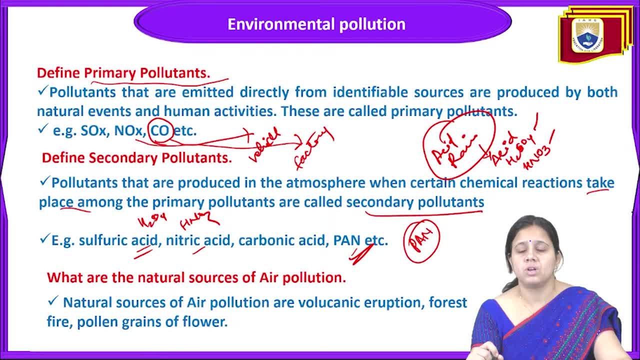 sources is also there. So the air pollution, natural sources, volcanic activities, forest fire and pollen grains of flower. So pollen grains of flower are the aero allergens. These are aero allergens That is present in the atmosphere. Then volcanic eruption, that is, volcanic activity, volcanic. 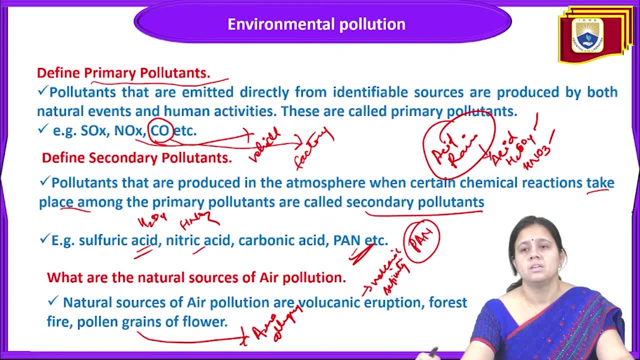 activity, Then forest fire. So these are the natural things that will be producing some pollution that will be harmful to the air. So they are the natural sources of air pollution. That is first. one is the volcanic activities, forest fire and pollen grains of flower- All 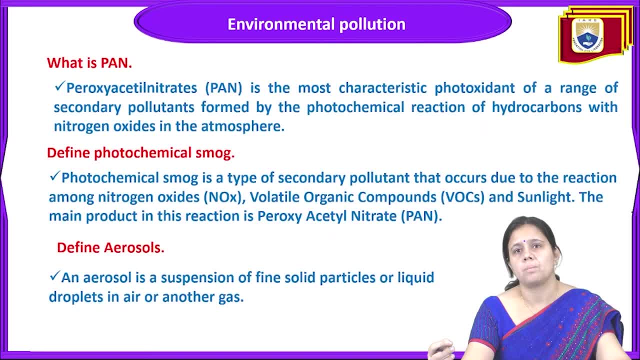 these are the natural sources of air pollution. Now comes to the next dimension. So the next topic, the next term, that is PAN. We have already discussed that. the PAN is a secondary air pollutant. So how this PAN is formed and what is PAN? PAN is a very important question, Like PAN is. 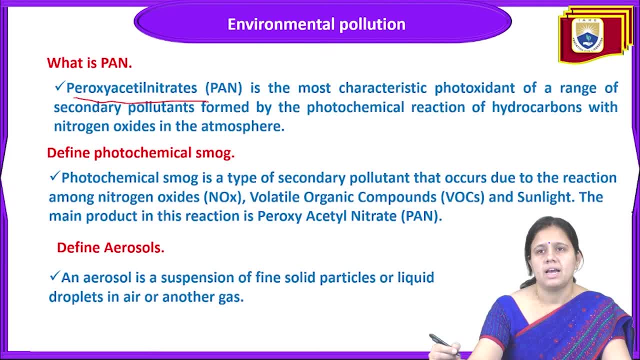 a. we can say that it is a peroxyacyl nitrate, and it is the most characteristic photo oxidants of a range of secondary pollutant that is formed by photochemical reaction of hydrocarbon with nitrogen oxide in the atmosphere Means. PAN is formed by the 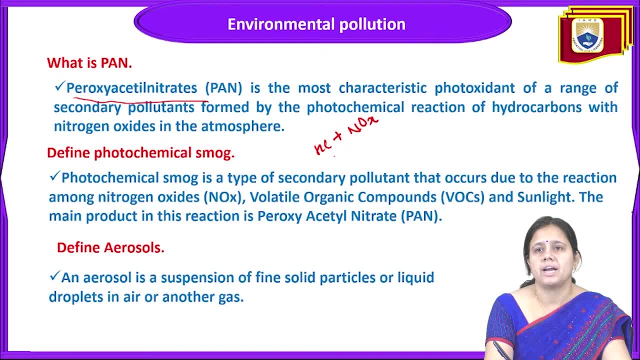 formation of hydrocarbons plus nitrous oxide means hydrocarbons is there. Hydrocarbons is a primary pollutant and NOX is also primary pollutant. that is, NOX is coming from vehicle pollutions, Hydrocarbons will get from combustion. So these two primary pollutant After reaction. 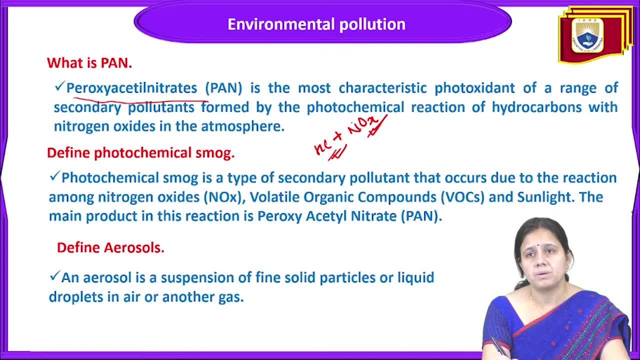 between these two primary pollutants: one, in the presence of photo oxidants, in the presence of sunlight, that some photochemical reaction will happen and that photochemical reaction will form one product that is peroxyate. This is a very dangerous pollutant and it is the most important secondary pollutant. 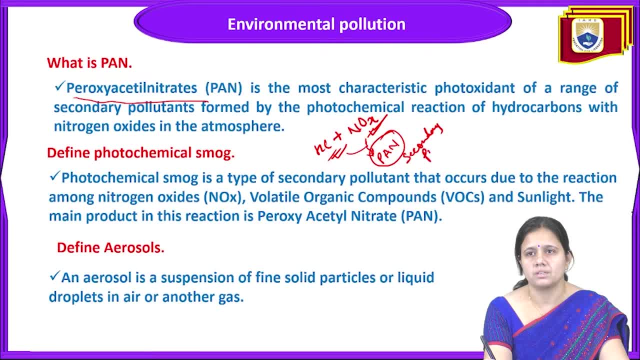 as we have already discussed about the secondary pollutant, This is formed by the reaction between two primary pollutants in the presence of photochemical reaction. This is called as PAN. So next is the defined photochemical smoke. As we have already known, smoke is formed by the two words smoke plus fog. 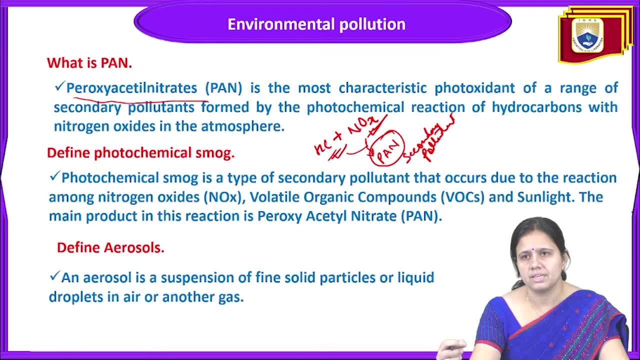 This is a very important term. in the air pollution. Smoke is equal to smoke plus fog. when there is a combination of smoke with the fog, that is called as smoke. So photochemical smoke is a type of secondary pollutant that occurs due to the reaction. 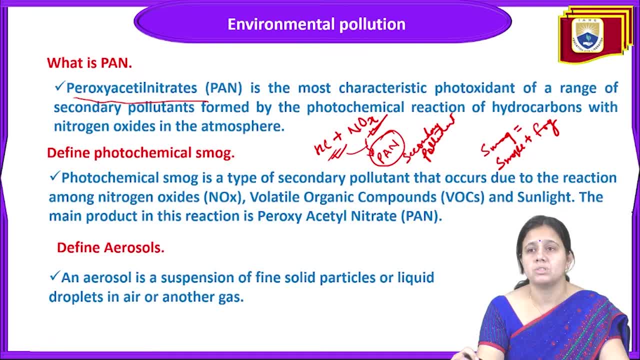 among nitrogen oxide, volatile organic compounds and sunlight. This photochemical smoke is a type of secondary pollutant Smoke is also a secondary pollutant Photochemical smoke. as the name suggests, photo means light. We already know photo is equal to light. So this photochemical smoke is a secondary pollutant and that will form due to the reaction. 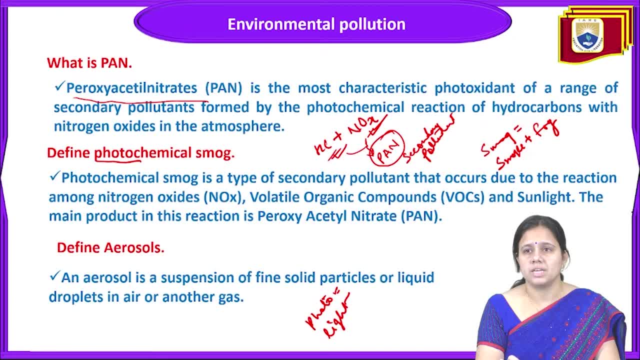 among nitrogen oxide, volatile organic compounds and sunlight, NOx. reaction of NOx with VOC In the presence of sunlight. that is why it is named as photochemical smoke, and the product will be formed is called as peroxyacyl nitrate. So PAN is responsible for this photochemical smoke pollution. 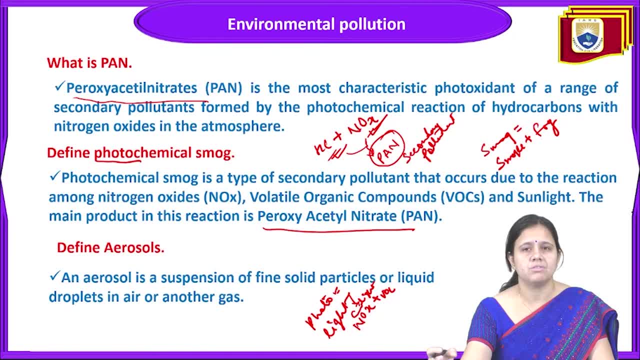 Smoke is a combination of smoke plus fog and it is a very dangerous kind of air pollution and it is a secondary air pollution. So how this photochemical smoke is all? this pan is all responsible for this photochemical smoke. Photochemical smoke is that type of secondary pollutant which occurs due to the reaction. 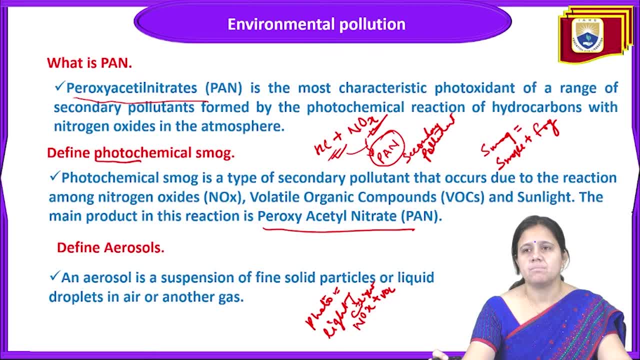 among the nitrogen oxide, volatile organic compounds and sunlight, and the product in this reaction is the PAN peroxyacyl nitrate. Next term is the define the term aerosol. aerosol is a suspension of fine liquid particles or liquid droplets in air or another gases. 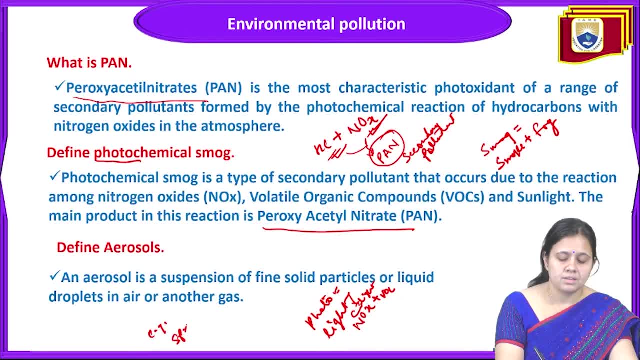 You can an example of it. It is a spray spray in tin can. This is a spray spray in tin can. This is a spray spray in tin can. This is a spray spray in tin can, And this is a spray spray in tin can. 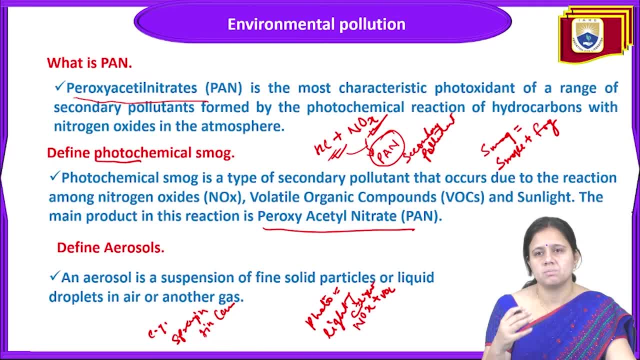 Is an example of aerosol. aerosol is nothing but a suspension of fine liquid particles or solid particle that is droplet in the air or another gases, as aerosol. aerosol is a suspension of fine liquid or solid that will be, that will be formed liquid droplet in the air or 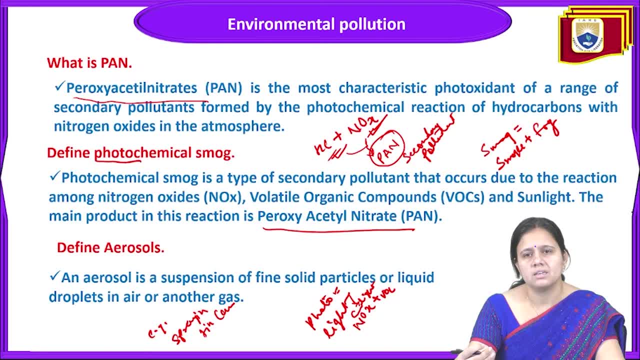 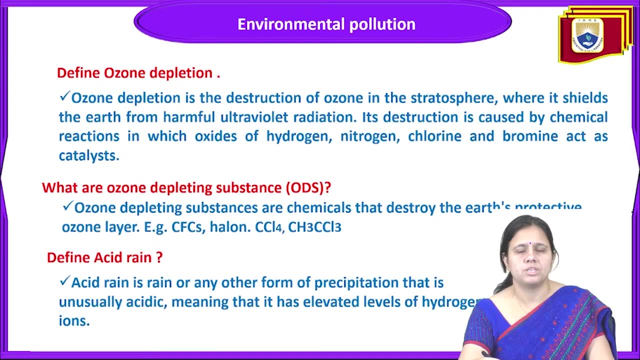 sometimes with the another gases called as aerosol, and example for this all we can say that is: the sometimes spray is there in a tin can is an example for this aerosol. next term is the ozone depletion. next, this is also related to the air pollution. what is ozone depletion? define the term depletion of ozone. ozone depletion is a very 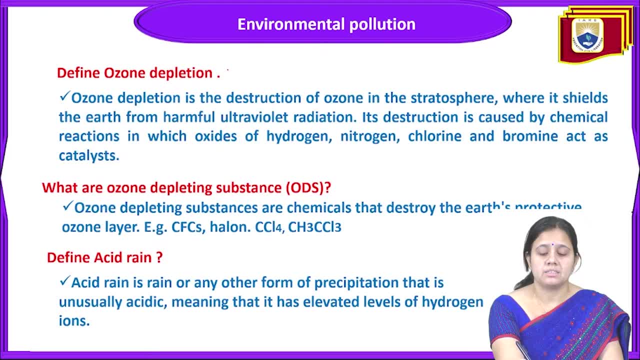 important question, and we can also term it as a thinning of ozone layer. thinning of ozone layer, ozone layer or sometimes a hole in the ozone layer, hole in ozone layer. so this all term is related with this. ozone depletion: ozone depletion is a destruction of ozone in the stratosphere where it shields the earth from harmful ultraviolet radiation. 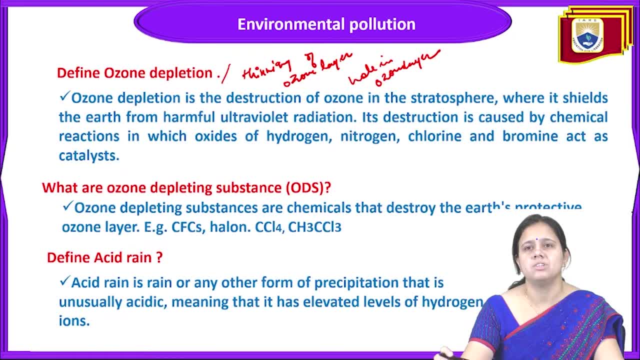 and this destruction is caused by some chemical reaction in which oxides of hydrogen nitrogen, chlorine and bromine act as a catalyst. so ozone depletion is nothing but a destruction of ozone layer in the stratosphere. in the stratosphere ozone layer is there and that destruction in the ozone layer, where it. 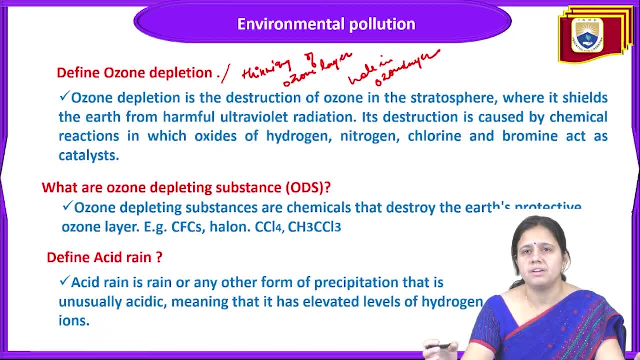 shields the Earth from harmful UV radiation where it will be mesmo. this ozone layer is present in the stratosphere. in the stratosphere you can see this is the stratosphere and one layers there. this layer is called as ozone layer and this layer is acting as a shield with the harmful UV radiation. 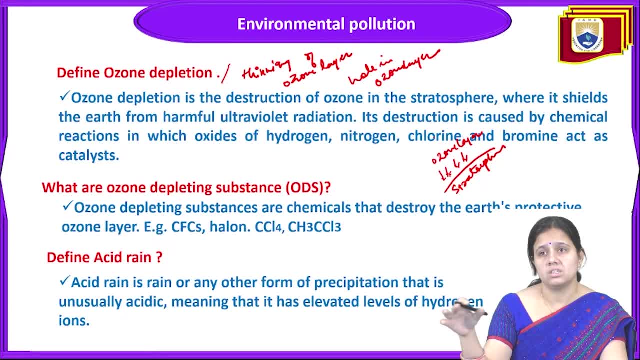 means many UV radiation there in and on the above the stratosphere. so what this ozone layer is do? they are acting as shield for this harmful uv radiation. so what will happen due to this air pollution? some cfc compound is there, chlorofluorocompound is there and that is causing the destruction of the ozone layer. 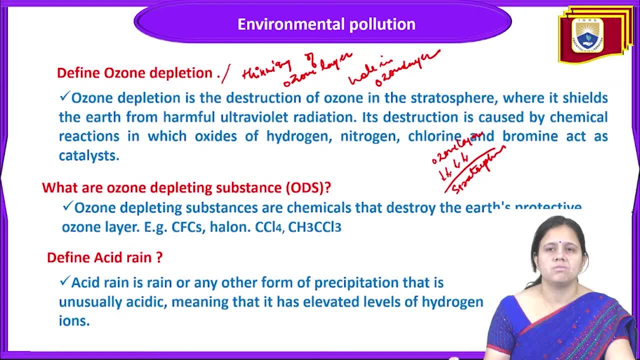 used by some chemical reaction and that chemical reaction will happen with the oxides of hydrogen, nitrogen, chlorine and bromine. that will be acting as a catalyst. sometimes this chlorine and bromine is acting as a catalyst and they are going to deplete the ozone layer that is present in the 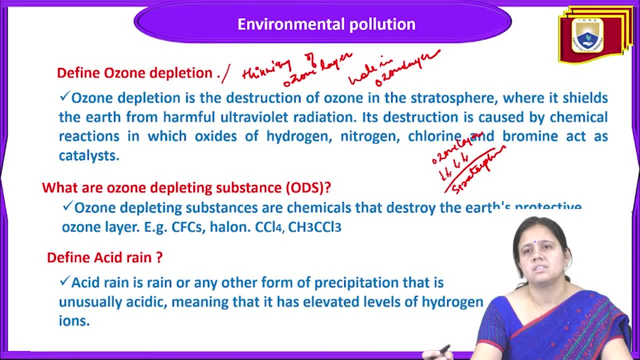 stratosphere. this is called as depletion of ozone is a destruction of ozone layer in the stratosphere. ozone layer: is there in the stratosphere? some destruction? is there? some hole is there that harmful uv radiation is causing, causing hole in the ozone layer that is causing? 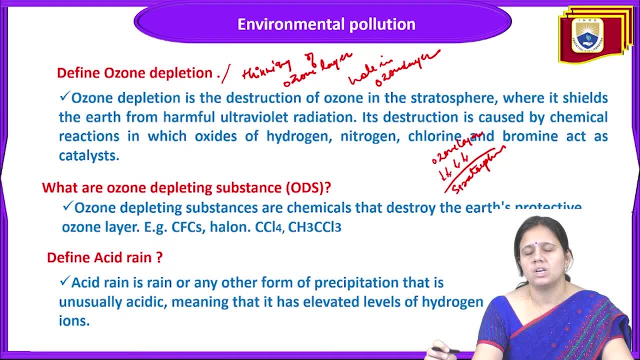 depletion in the ozone layer and due to this, ozone layer is getting destructed, and it is this. destruction is caused by the chemical reaction which will be happen with the oxides of hydrogen, nitrogen, chlorine and bromine. all are acting as a catalyst in this ozone layer. destruction- and this ozone layer is basically destruction- is 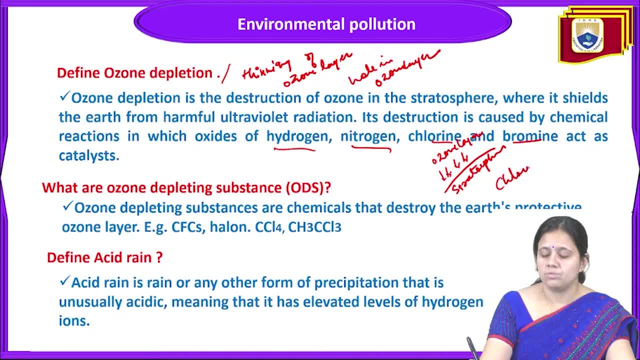 basically caused by the chlorofluorocarbon. chlorofluorocarbon, as we have already discussed in the lectures, chlorofluorocarbon, cfc, is there. cfc is originating from our refrigerators. it is all this. cfc is originating due to human. 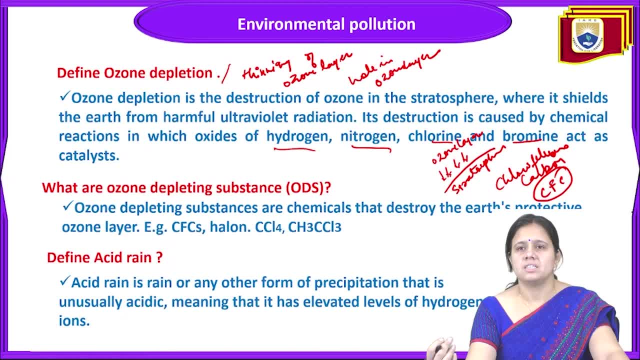 activity due to this is anthropogenic. and next is the. what is ozone depleting substances means, what are the substances that is depleting this ozone layer? which substance is responsible for the depletion of ozone layer? so, ozone layer depletion are the substances there. they have. 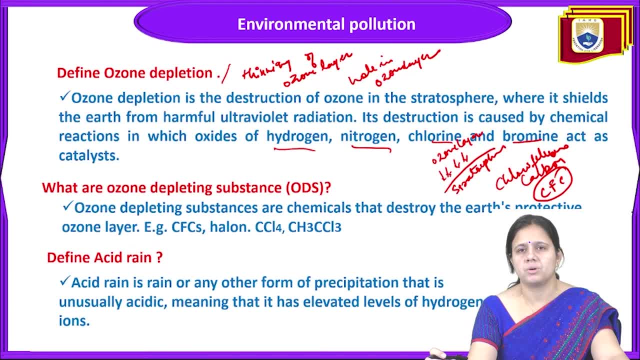 some chemical reaction that destroy the earth's protective ozone layer. some chemical reaction will be happen in the stratosphere and some gases will be formed, like cfc, halones, chlorofluorocarbon, cs3, ccl3. so these substances will be formed in the atmosphere and these substances is 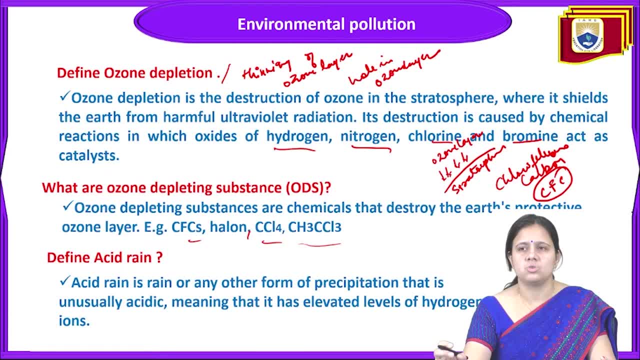 all due to the some chemical activity that will destroy the earth's protective layer that is called as ozone layer. depletion is caused by chlorofluorocarbon and halos that are originating due to the industrial activity, anthropogenic activity and human activity and refrigerator fire extinguisher ac. we are using. 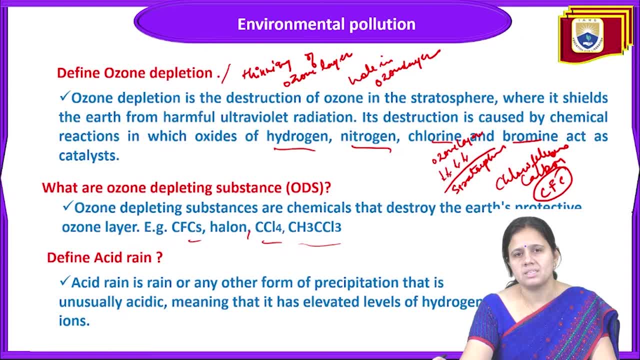 so with all these electrical appliances, this kind of gases is originating in the stratosphere and in the stratosphere they are depleting the ozone layer that is acting as a against the some uv rays and some very dangerous, harmful ultraviolet rays. next question is about acid rain. acid rain, what is acid rain means? what is acid rain? we can say? 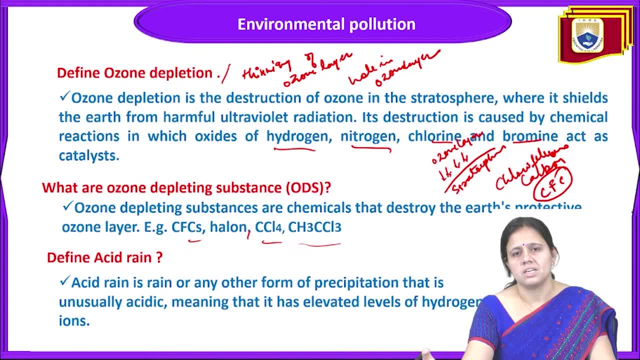 that rain water that is acidic in nature is called as acid rain, if we will understand this term in a very general manner. like rain, water that is containing some harmful concentrated acid is called as acid rain, acid rain is a very dangerous and harmful acid rain. acid rain is the rain or any other form of precipitation that is usually acidic in nature. 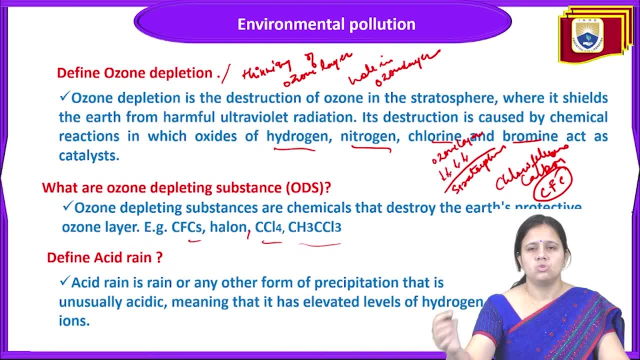 means that it has elevated level of hydrogen ions means those rains, h2o is there and that will be mixed with some um. with the reaction that will be some acid will be there in the rain water. that is called as acid rain. so what will happen if, with the h2o is there, water is there, with the reaction. 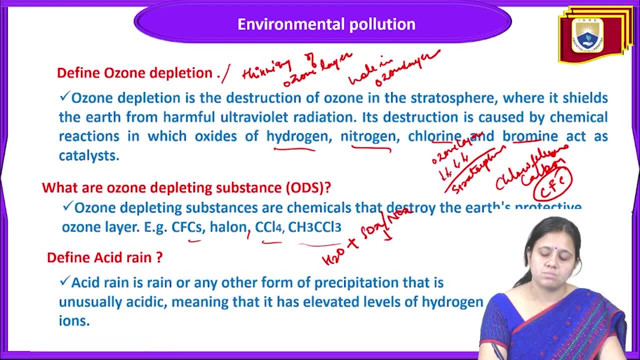 between socks or knocks to next product will be formed. this product is either h2, so4 or hno3, so h2so4 means water, is there? some socks and knocks will be originating due to vicular pollution with vile pollution, automobile pollution or by some, uh, industrial activity. so these socks and knocks will be formed and these 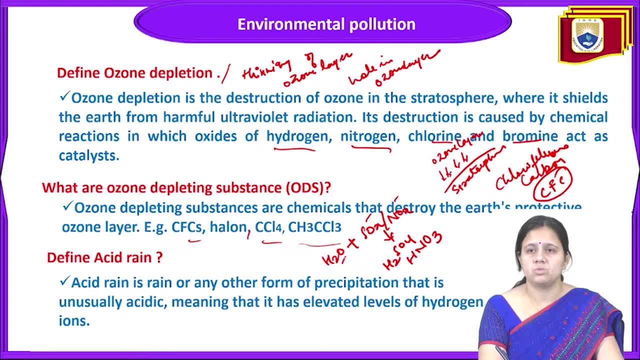 two primary pollutant will form reaction with h2o and then two type of secondary pollutant will be formed. that is first. one is the h2o and then the second one is the h2o. then a very dangerous active is first. one is the h2so4, and hno3 means rain water containing high concentration of h2so4 or 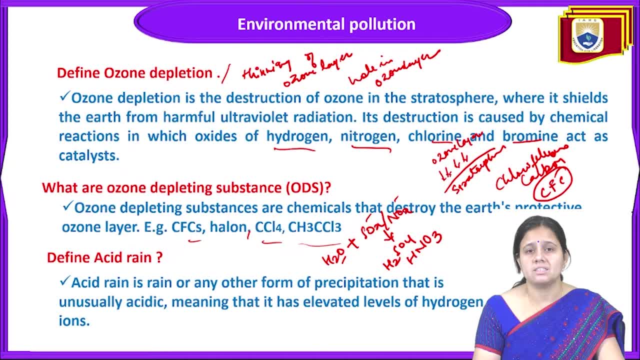 hno3 is called as acid rain and this acid rain is corroding, corroding the surface of taj mahal and it is a very important case study that is related with this acid rain. this is called as acid rain means those rain that are that are usually acidic in nature is called as acid rain. 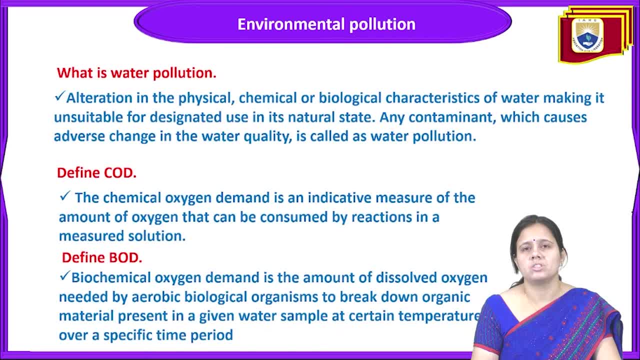 now a next question. next terminology related with this topic is the define the term water pollution, water pollution. we can define water pollution as the in alteration in the physical, chemical and biological characteristic of water that will be unsuitable, unfavorable for the designated use, in the natural state or any contaminants which causes adverse change in the water quality is. 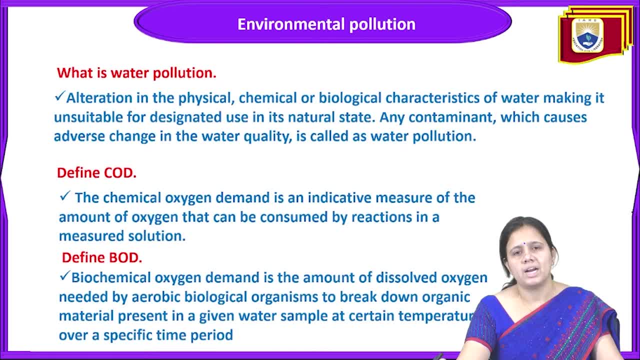 called as water pollution means alteration or undesirable change in any physical, chemical or biological characteristics of water that will be unsuitable or unfavorable for the use for the water and that will be harmful for the living organism is called as water pollution so we can define. water pollution is like any 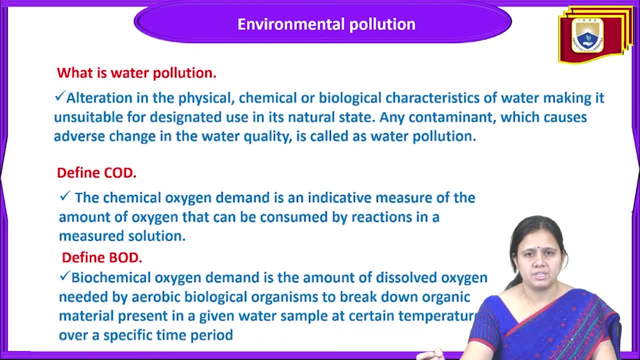 undesirable change in the physical, chemical or biological properties of water and that will be undesirable, that will be unsuitable for its use, is called as that that will be harmful for human being or any. any living organism that is associated with the use of water is called as water pollution. 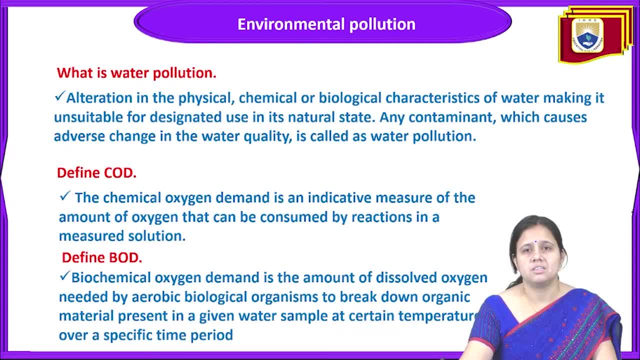 next term related with this. water pollution is a define the term cod, chemical oxygen demand. cod means chemical oxygen demand. chemical oxygen demand means basically this two: what is related with the water pollution means? first one is the chemical oxygen demand. it is an indicative measure of the amount of oxygen that can be consumed by reaction in a measured solution. means what will happen. 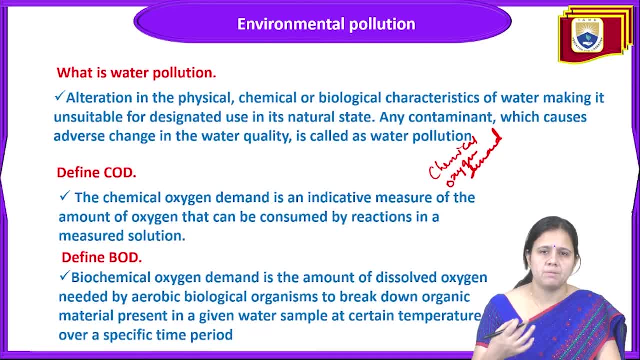 chemical oxygen demand means the demand of oxygen by any microorganism for their activity, for their activity to decompose the decompose, the organic material that is present in the water, that is that organic. is the water pollutant? organic is there? organic substance is there that is water. 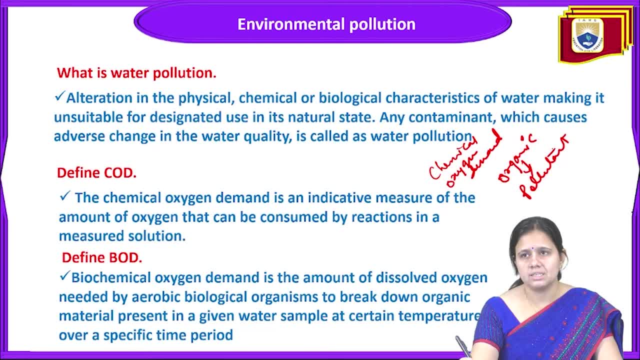 polluted. so the amount of oxygen that is needed by the particular organism to degrade that organic material into the water is called as chemical oxygen. demand means that demand of oxygen, that amount of oxygen that is needed by an organism, by a microorganism, to degrade the, degrade the organic. 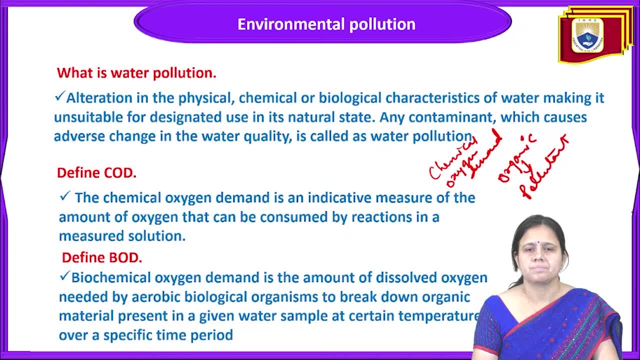 materials in the water is called as chemical oxygen demand means oxygen demand for the chemical activity by the microorganism for the degradation of organic materials that is present in water is called as chemical oxygen demand. so we can understand water pollution by these two things: cod and pod. cod is chemical oxygen demand. bod is biological oxygen demand. 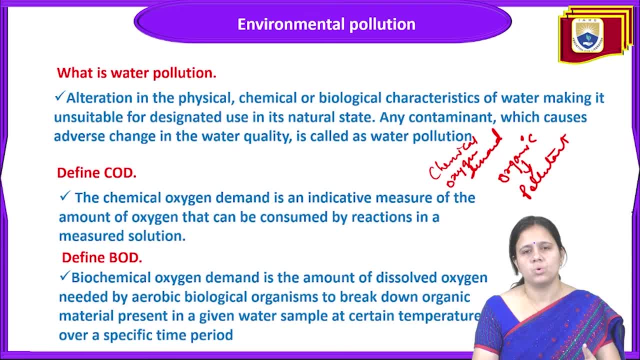 so, cod, if the amount of oxygen demand is more by the microorganism, that means the pollution is more organic material is more. so this is an indicative for the, the water pollution. we can say that will be an indicative term for the water pollution. next point is related with the water, is the bod. bod is the biochemical oxygen demand. it is. 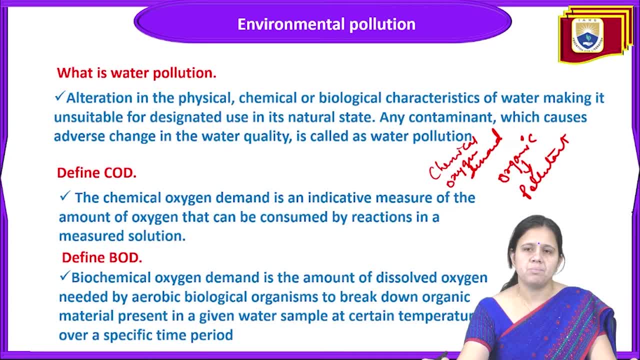 again, the amount of dissolved oxygen needed by the aerobic biological organism to break down organic material present in a given water sample at a certain temperature over a specific period of time is in five days. five days and 20 degrees celsius. this is the basic criteria for this. 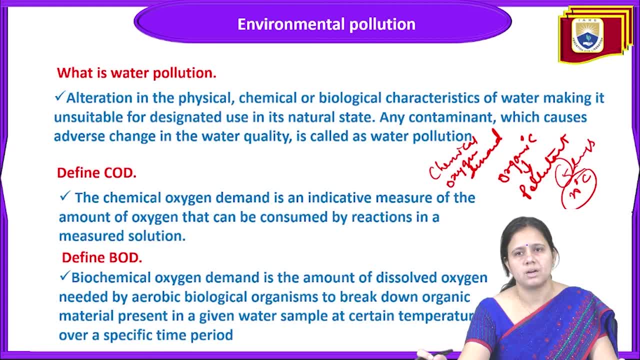 biological chemical oxygen demand. bod- biological oxygen demand. so that amount of dissolved oxygen that is needed by an aerobic bacteria, aerobic organism to break down organic material into the given water sample at certain temperature or over a specific time period, is called as bod. bod is the amount of dissolved oxygen that is. 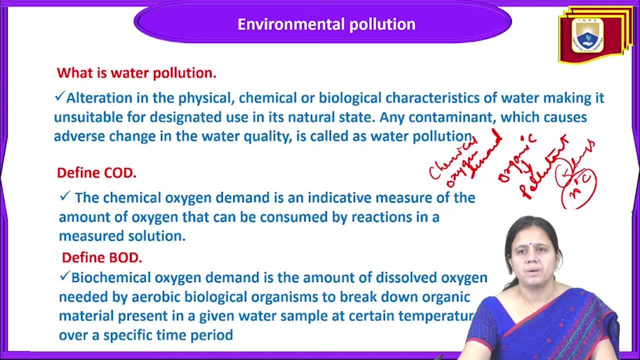 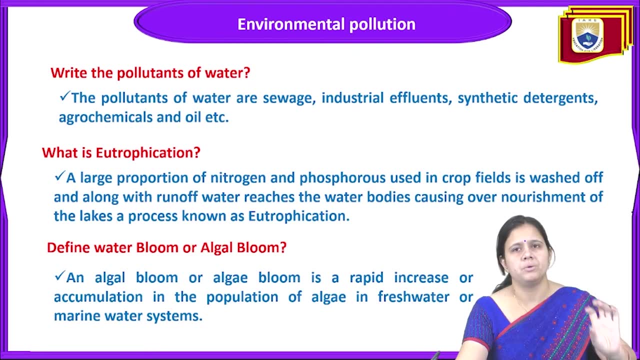 needed to break down organic material into the given water sample at a certain temperature over a specific time period is called as bod. next is the. what are the pollutant of water, as we have already discussed like what does it mean by pollutant? pollutant are those agent. 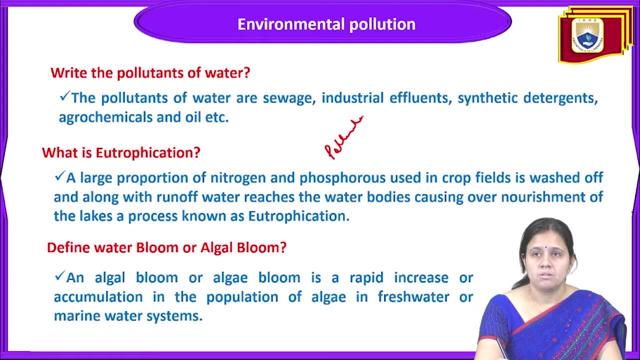 that is causing pollution. pollutants is equal to those agents. those agents that are causing that, are causing that, are causing pollution. pollution is called as pollutant. so the pollutant of water is the some sewage is there. industrial effluent, synthetic detergent, agrochemicals and oil means sewage is there that is dirty water, that. 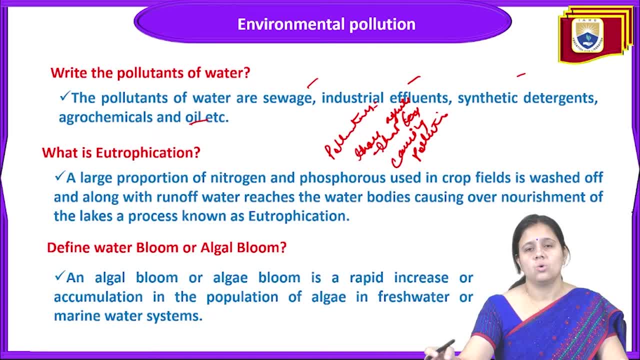 that is, water that is originating from our daily activity, is called as sewage. so sewage is there and tastkle affluences. industrial effluent means affluent that is throwout from the industries. next is a some synthetic detergents we are using for our washing purpose. agrochemicals means those pesticides. 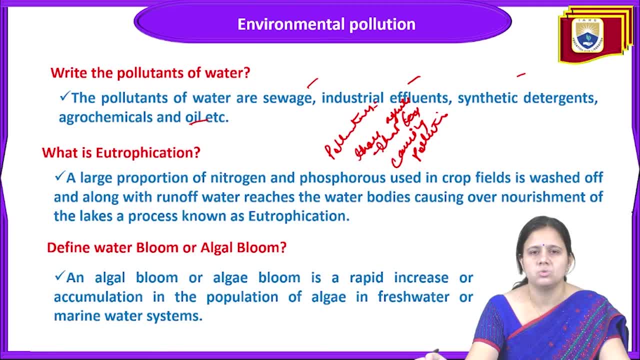 or chemical substances, chemical fertilizers, that is, that are using in the agriculture activities. next is the oil. they are the common air pollutant, water pollutants. they are the main water pollutants. next term is the what is back to the sun and come back the next morning. even water volumes and plastic había. 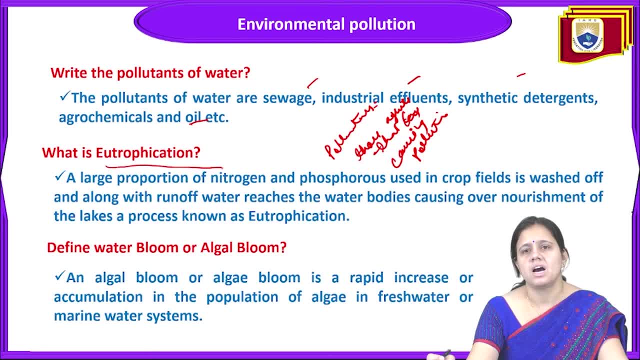 eutrophication. eutrophication is the large proportion of nitrogen and phosphorus used in the crop field. it is washed off and, along with runoff water that reaches the water body and that nitrogen and phosphorus will causing over nourishment of the lake, is known as the 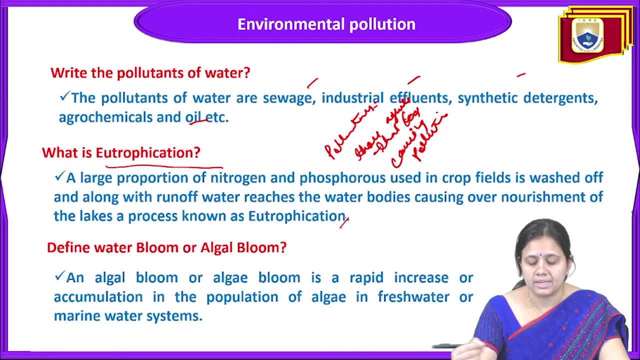 eutrophication lake. that lake is called a eutrophic lake, eutrophic lake, eutrophic lake. so a large proportion of nitrogen and phosphorus is used in the crops in the agricultural activity and then that will be washed off along with runoff water and that reaches the water bodies. that is. 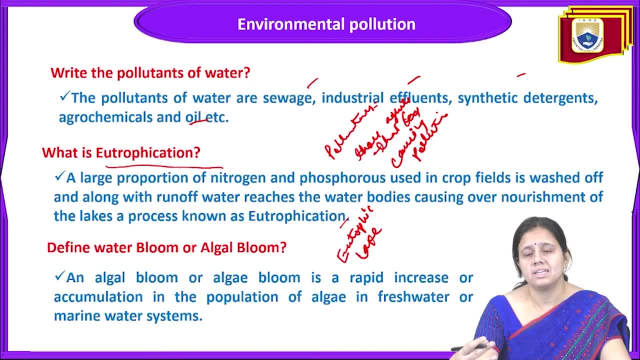 causing over nourishment of the over nourishment of the lakes, and the process is called as eutrophication. next is the term that is related with this eutrophication, that is, algal bloom or water bloom. this is a very important term that will be asked in many examination, like: what is algal bloom or water? 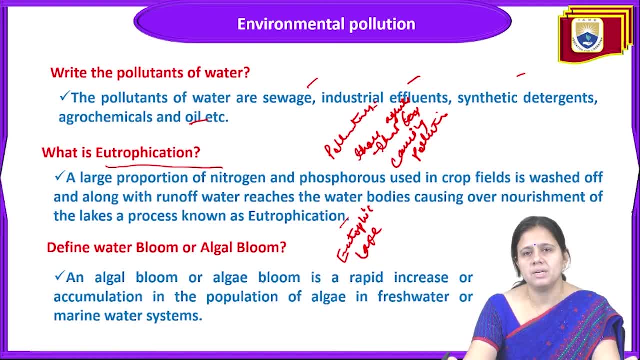 bloom. algal bloom is the bloom of algae. that is rapid increase or accumulation or population of algae in fresh water on long-time marine water system. so due to the runoff from agriculture runoff, extra nitrogen and phosphorus will enter into the water and that will be provided. 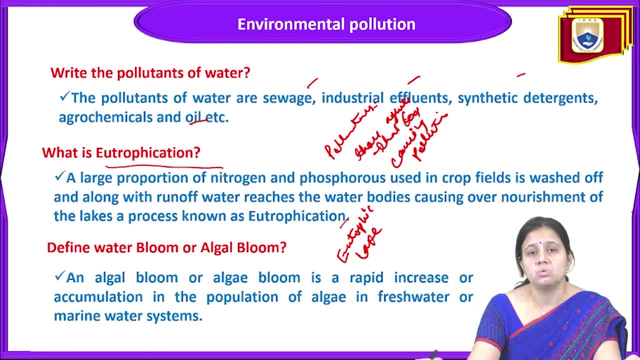 nourishment to the algae that is already present and due to more nourishment some excessive growth and rapid growth of the nutrient sap does not need to be demoed. but as we call ash, called fast encirclement and it takes time and because we are talking about both margin and the basic shrimp, we i had differentuju to method. 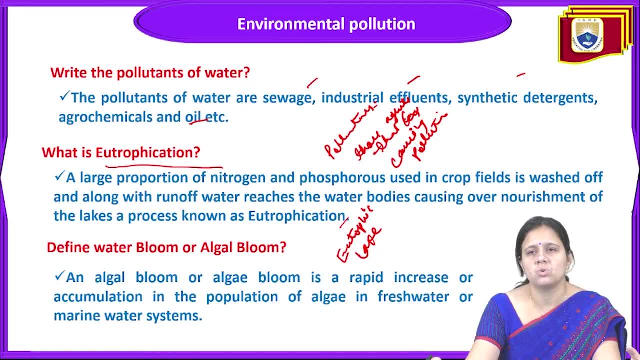 of the algae is there and due to this population growth, algae, fresh water and marine water system green color is there. that is called as water bloom or algal bloom. that is the, if we understand in a basic term like more rapid increase in the accumulation of population of algae. 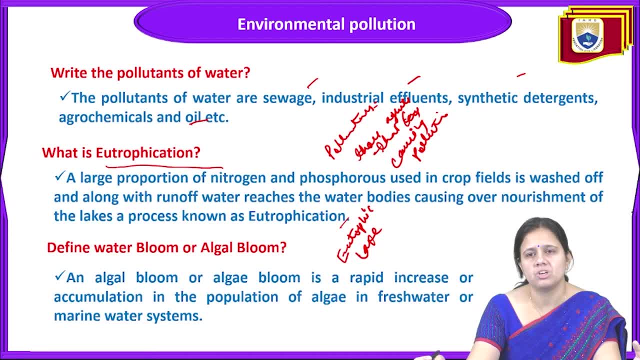 is called as algal bloom. means more increase in the population of algae, is known as algal bloom and algal bloom means sometime it will happen in fresh water or sometime it will happen in marine water. means the excessive growth or rapid increase in the accumulation of the 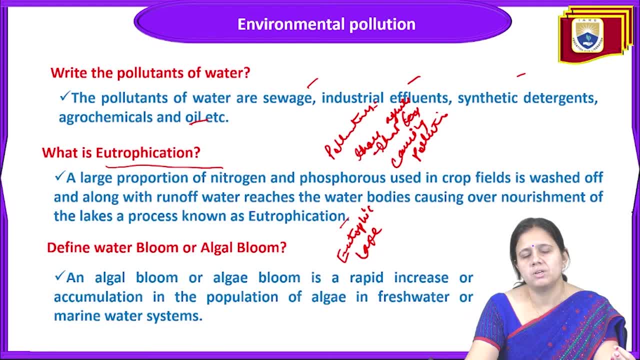 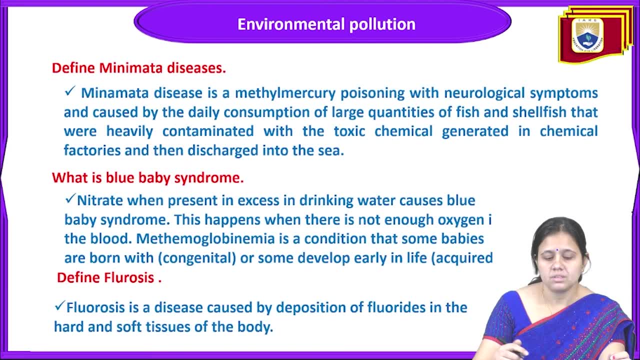 population of algae due to some nutrients, over nourishment of, due to some nutrient like nitrogen and phosphorus, that is called as algal growth or algal growth, now the term mini mata disease. mini mata disease is the disease that is caused by methyl mercury. methyl mercury- ch3- hg. 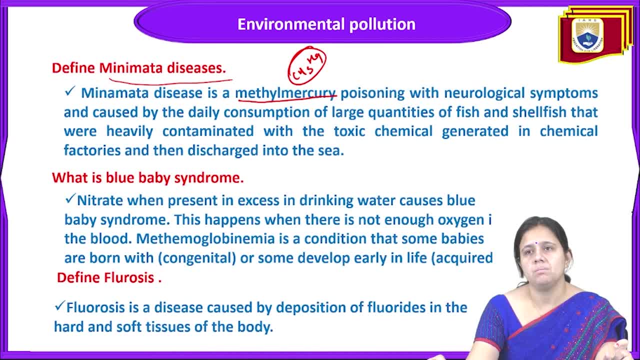 is there and what will happen? this methyl mercury is a very poisonous and with the neurological system is there, and it is caused by daily consumption of large quantities of fish selfish that were heavily contaminated with the toxic chemicals generated in chemical factories and then discharge into the sea. this is again a case of we have already talked about. 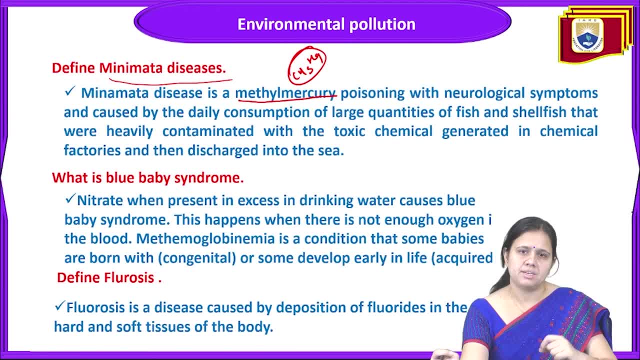 biomagnification. due to biomagnification of chemicals into the fishes and then fish eaten by the man, methyl mercury will enter into the human body and this methyl mercury is a very dangerous substance that is causing poisoning with a neurological system symptom and caused by daily consumption of large quantity of fish, seafoods, and that that fish and seafood will be contaminated. 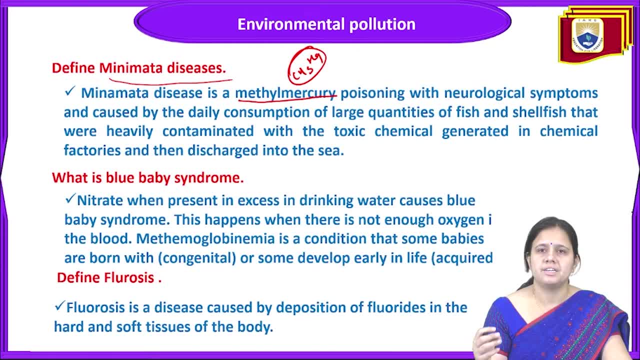 with the toxic chemicals and this chemical is generated from the factories and they are direct discharging this chemical directly into the sea. due to this activity, this methyl mercury will enter into the fish body and the person who are consuming the fish at a large amount or in daily intake. maybe that person will be affected by this. 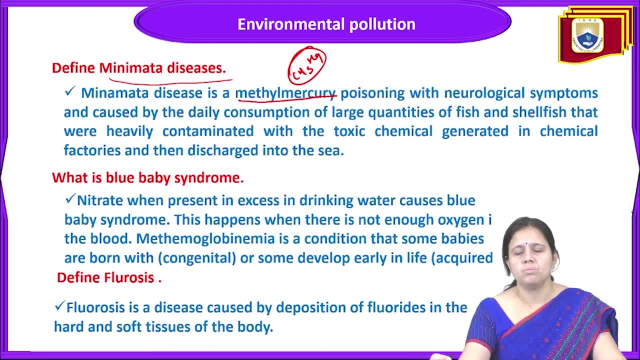 minimata. this next is the blue baby syndrome. blue baby syndrome is due to the nitrate nitrate. when nitrate present in excess in the drinking water, that is causing blue baby syndrome. this will happen when there is not enough oxygen into the blood and one condition will be formed: that 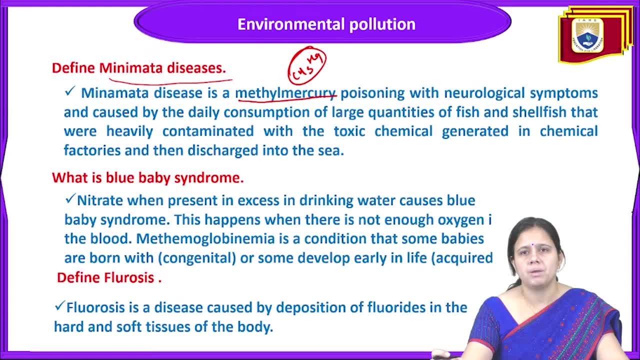 as methamnoglobinemia is a condition that some baby are born with cognitin or some develop early in life. what will happen? nitrate if, due to drinking water, nitrate is there in water. when, when excess of nitrate is in water, that will be causes to infants that their nitrate amount in the body. 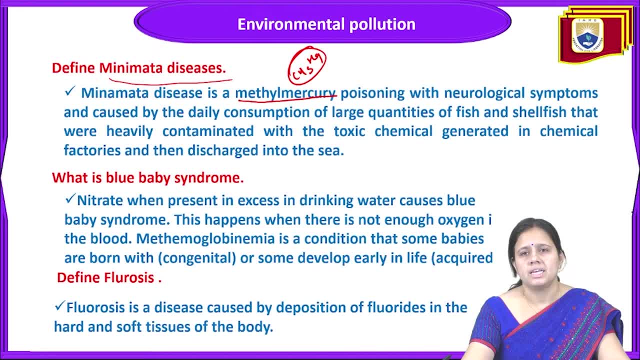 is increases and there is not enough oxygen in the blood. in this way, the body is turned totally blue. this is called as blue baby syndrome and the condition will happen, will form like methamnoglobinia condition is there in which some baby are born with subcognital issue or they have developed some. 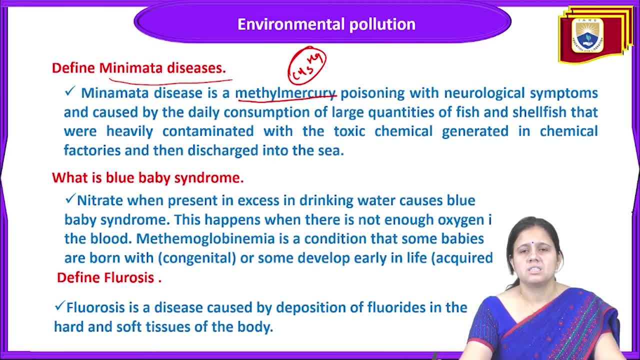 early life activities. next is the term, that is, fluorescence. fluorescence is caused by deposition of fluorides in the hard and soft tissue of the bone, and all these diseases are related with the water pollution, only due to water pollution only. so fluorescence is happened by by drinking water, which will contain fluoride. fluoride is there if drinking. 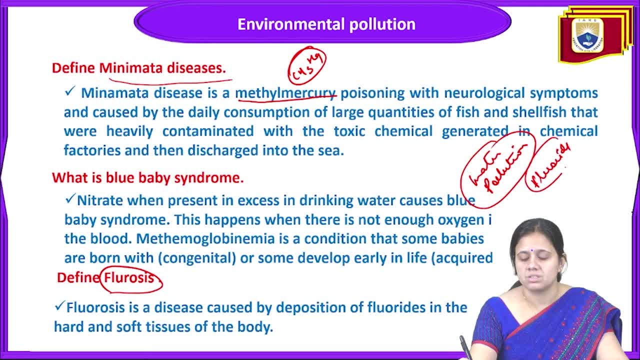 drinking water fluoride is present in more amount, then fluorescence condition will be formed and it is a deposition of fluorides in the hard and soft tissues of the body. on the hard and soft tissues of a human body, this fluoride is deposited, and all due to the drinking of dirty water, water containing 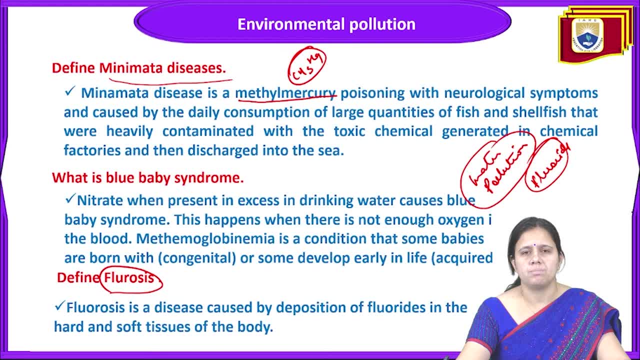 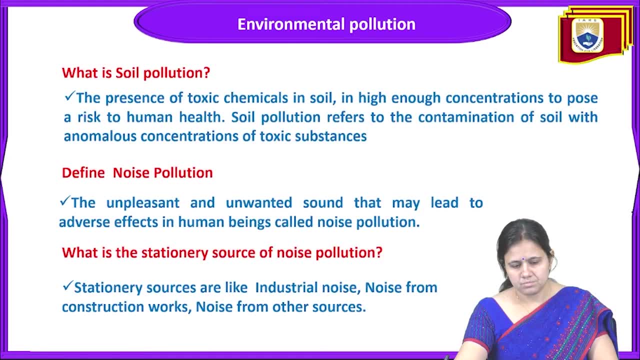 fluoride. see, this kind of condition will be formed on the fifth of a pimple. you can see that yellow, yellow, yellow. what is there? this is the reason. this is the symptom of fluorescence. now, next is a term related with the pollution of soil pollution. what is soil pollution? soil- 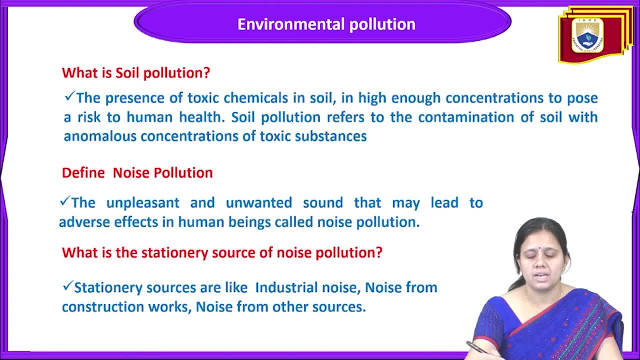 pollution is a presence of some toxic chemicals in the soil in high amounts that were in high concentration to pose a risk to human health, and this soil pollution refers to the contamination of soil with anomalous concentration of toxic substances like toxic metal, heavy metals, toxic metals like arsenic, mercury, mercury, zinc. 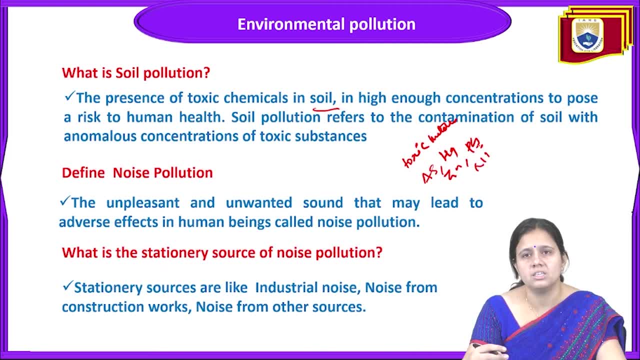 lead, nickel- all these toxic chemicals will enter into the soil and that will be risk for human health- is called a soil pollution. presence of any toxic chemical in the soil in a more concentration that will be causing risk to a human health is called a soil pollution. soil pollution refers 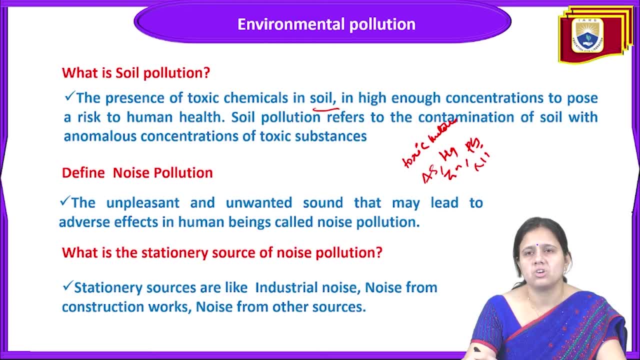 to the contamination of soil with anomalous concentration of toxic substances is called a soil. next term is the noise pollution. what does mean by none term noise pollution? so the unpleasant and unwanted sound that may leads to adverse effect in the human body is causing, as noise pollution means the pollution of noise like unpleasant or unwanted sound that may leads. 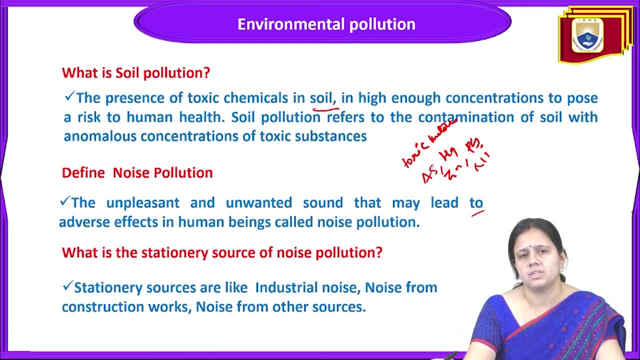 to adverse effect like. sometimes it will affect to the central nervous system, sometimes it will. it will cause the heart attack. heart pain is there. so the noise, that is more amount that will be unbearable or unpleasant, that will be unwanted and that will be causing some bad effect in the 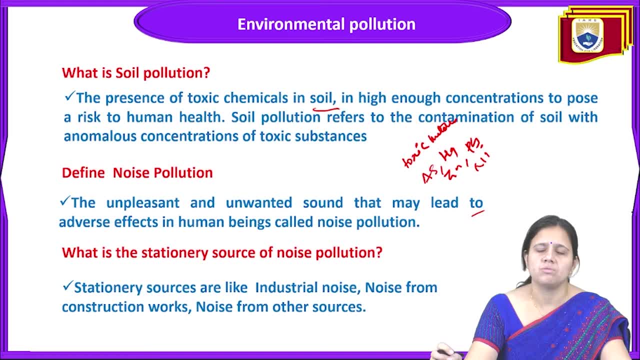 human being is called as noise pollution. so noise, for sources of noise pollution, is of two type. first one is the stationary source and then mobile source. stationary source is that source that are like that are present at the one place, and mobile source is like those sources that is. 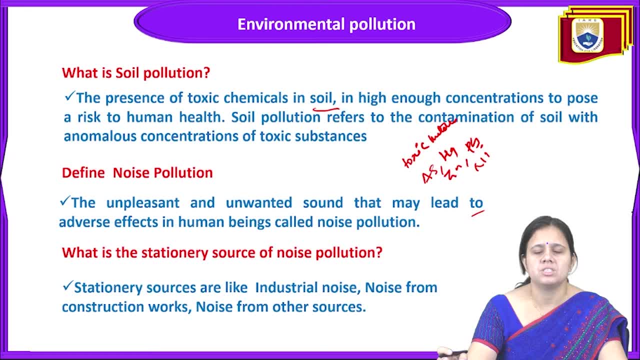 moving. so the stationary source, the example for stationary source, are like some noise from the industries, noise from construction activity, noise from some as sources. that source is already there means any high work, high construction activity. these kind of sources is called a stationary source and mobile source means those that is like horns from vehicles. you can say that this is a mobile source of noise. 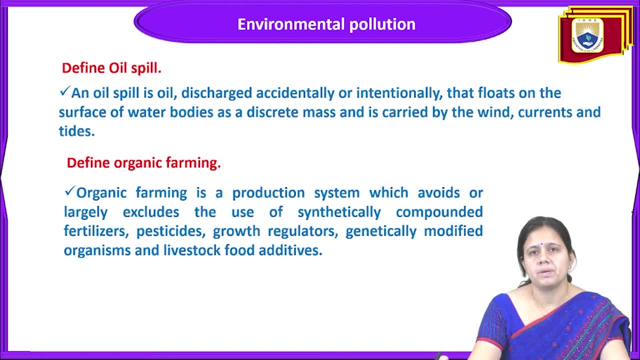 pollution. now next topic is the next term is the define the term oil spill. so oil spill is again related with the water pollution or sometimes soil pollution. so oil spill is a discharge of oil, uh accidentally or intentionally, that float on the surface of water bodies as a discrete. 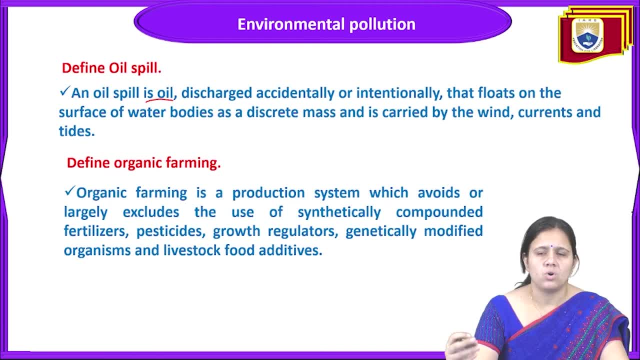 mass and is carried by wind, currents and types. oil spill is a discharge of oils into the aquatic system, sometimes in a marine system, sometimes in a marine system, sometimes in a marine system system also, and that will be present and the float on the surface of water as a discrete mass. 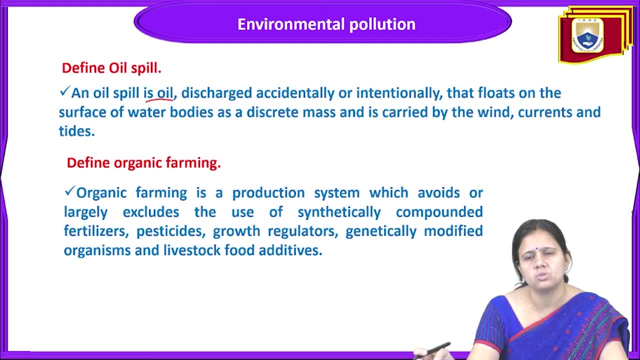 and it is carried by wind and ocean currents and wind ties to one place to another place and this oil spill sometimes. what will happen? due to this? um transportation of oil on the large, on the large boat, some spill is there and due to this spill, that oil is present in the water and